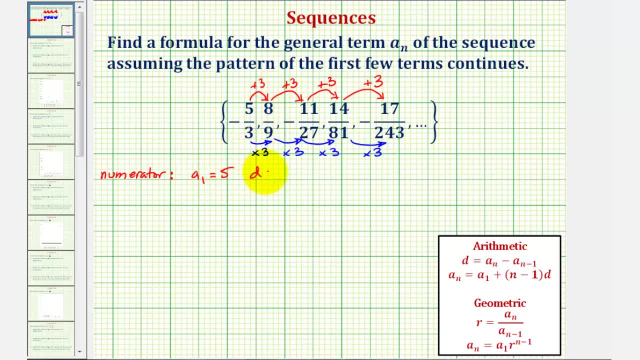 And then we'll find the denominator. And the common difference. d is equal to positive 3.. So using our formulas for an arithmetic sequence for a sub n, we can say that a sub n equals a sub 1,, which is 5, plus the quantity n minus 1 times d, which is 3.. 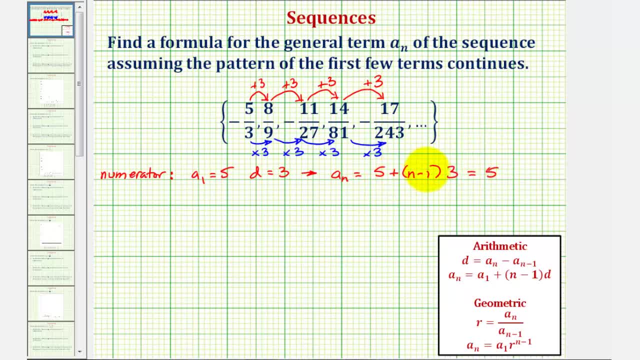 So let's simplify this. We'd have 5 plus 3n minus 3.. So just for the numerator, we can say that a sub n is equal to positive 3.. And then we'd have: 5 plus 3n is equal to 2, plus 3n. 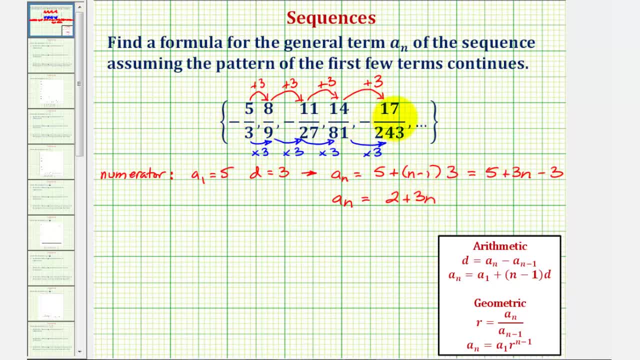 And now let's focus on just the denominator. again, ignoring the sign For the denominator, we can say that a sub 1 is equal to 3.. And r, the common ratio would be 3 as well. So now, using our formulas for a geometric sequence, here a sub n is equal to 3.. 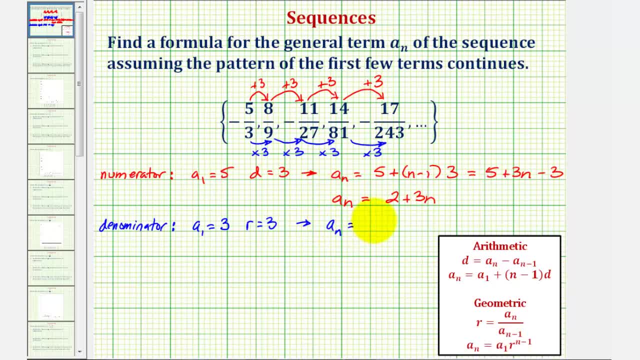 A sub n is equal to a sub 1,, which is 3, times r, raised to the power of n minus 1,, which would be 3 to the power of n minus 1.. Because a sub 1 and r are the same, we can multiply. 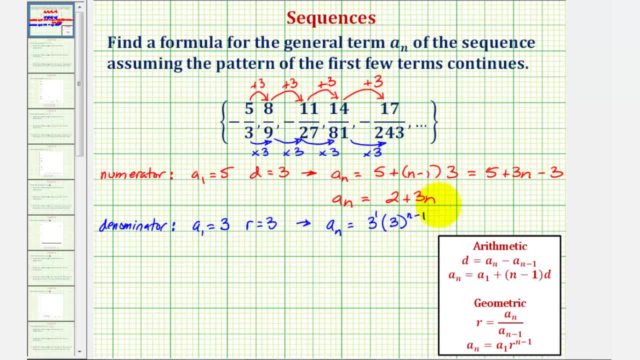 And when multiplying the bases are the same, we add the exponents- So this simplifies nicely- to just 3 to the power of n. So now, except for the alternating sign, we have a formula, a sub n, for the sequence A sub n would be equal to. again we can use the formula 2 plus 3n for the numerator. 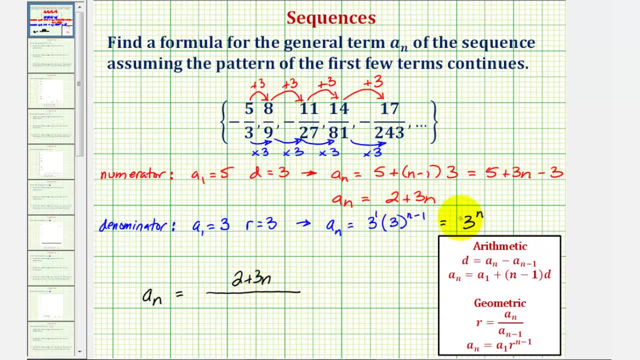 And we can use the formula 3 to the power of n for the denominator. But we still have to alternate the sign of the fractions And we can do this by using a factor of negative 1.. Notice how, if we multiply the numerator by negative 1 to the power of n, if n is odd. 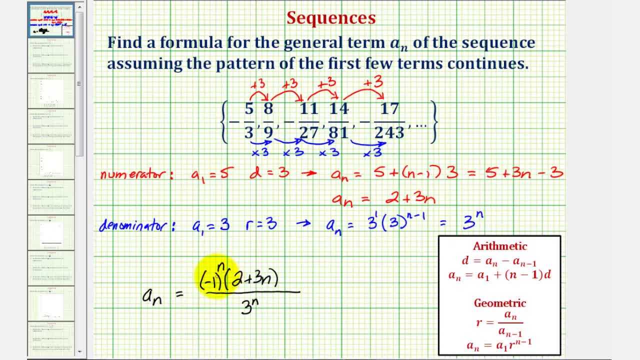 the fraction would be negative. If n is, even the fraction would be positive. Let's see if this works. Notice how the first, third and fifth terms are negative And the second and fourth terms are positive And therefore negative. 1 raised to the power of n would give us the correct sign.